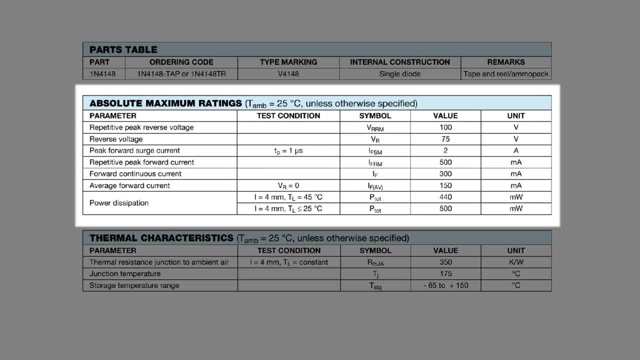 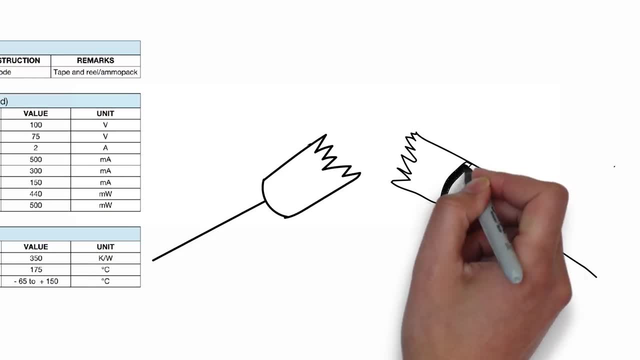 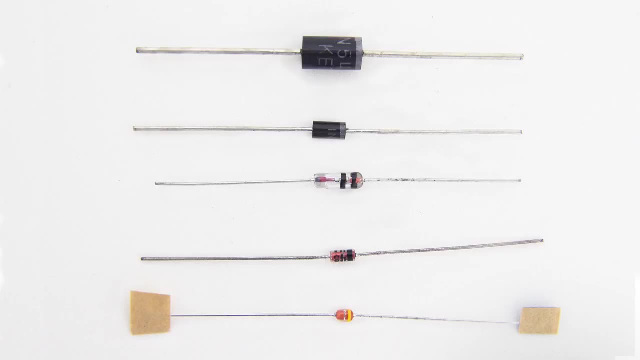 can withstand. The data sheet also indicates the maximum current ratings. Make sure your diode isn't exposed to more than these ratings or you'll risk permanently damage the diode. There are lots of different kinds of diodes. Let's go through some of the most common ones. 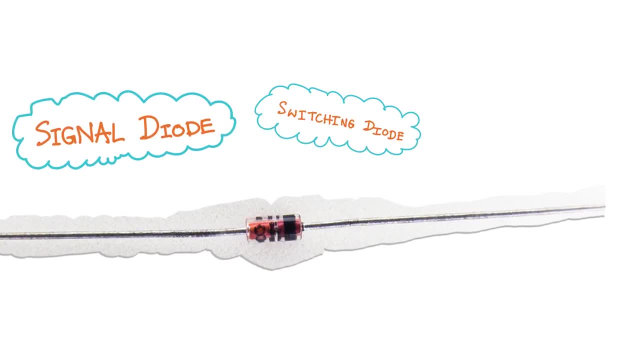 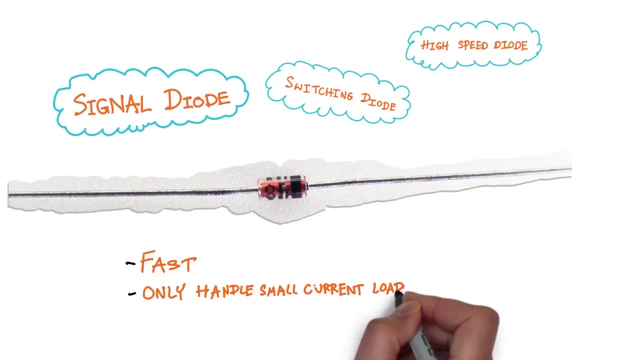 Signal diodes, Also known as switching diodes or high speed diodes. These type of diode are designed to be fast but can only have a maximum current of five volts per second. They can handle small current loads. The most commonly used is the 1N4148, and 1N914. These 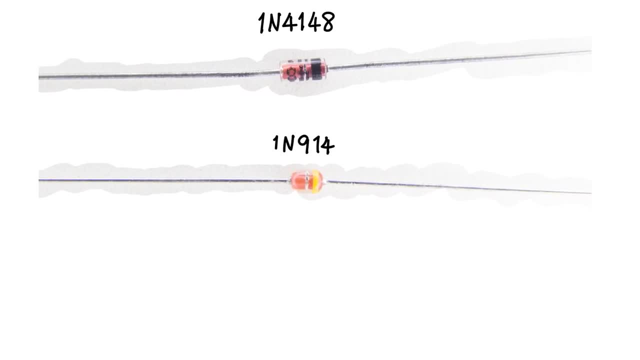 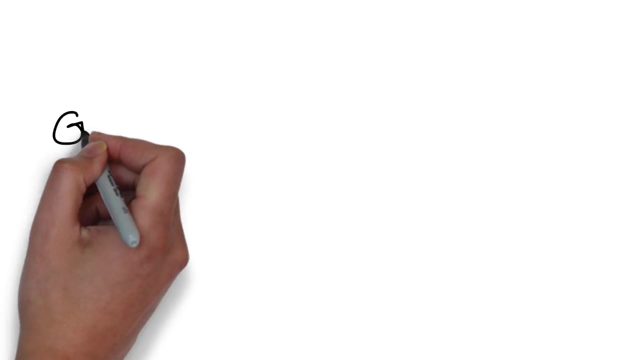 two diodes are quite similar and can be used interchangeably. They have a forward voltage drop of zero point six volt and peak reverse voltage of one hundred volts. They can carry a maximum current of two hundred milliamps. Some of signal diodes are made of germanium. 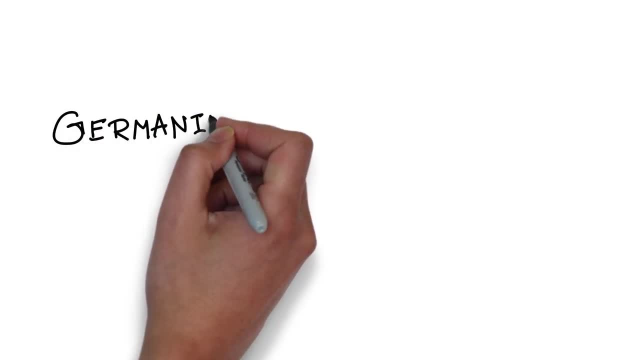 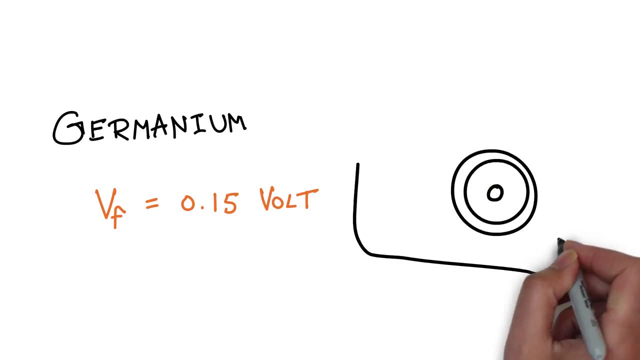 instead of silicon and they have much smaller forward voltage drop than the normal diodes. Some of these diodes are made of silicon and silicon diodes, and that can be as low as zero point one, five volt. They come in handy for some radio applications, which often 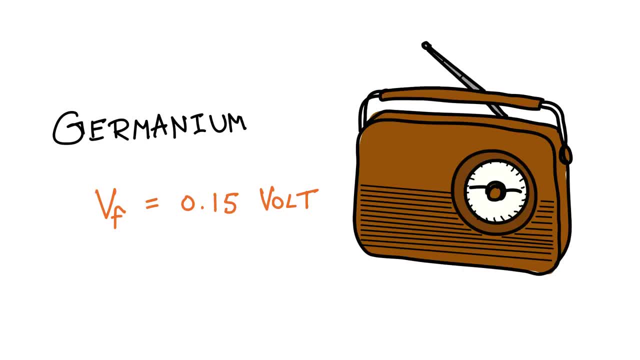 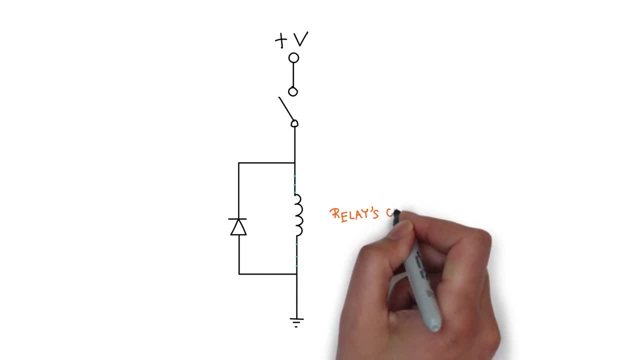 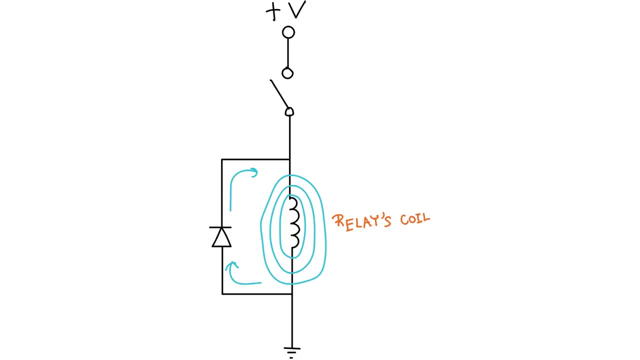 deal with very weak signal. Signal diodes such as the 1N4148 often find themselves used with inductors or relays to protect surrounding circuits from voltage spikes that can occur when the power to the inductor suddenly shuts off. Rectifier diodes. 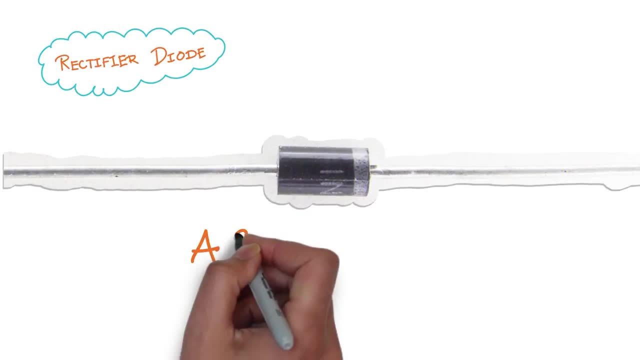 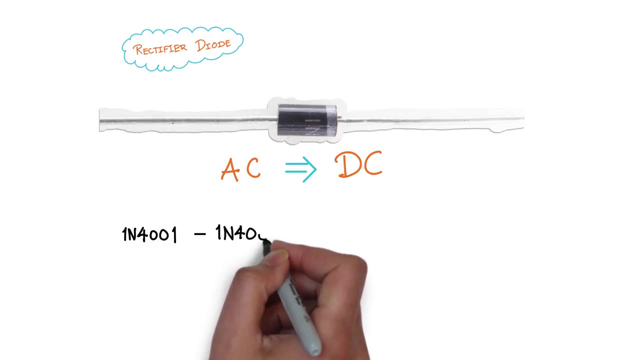 This is the type of diode you use when you want to convert alternating current into direct current. The most common ones are 1N4001, to 1N4007.. They can handle higher current- up to one amp. Their peak reverse voltage range from 50 to 1000 volts In household mains. 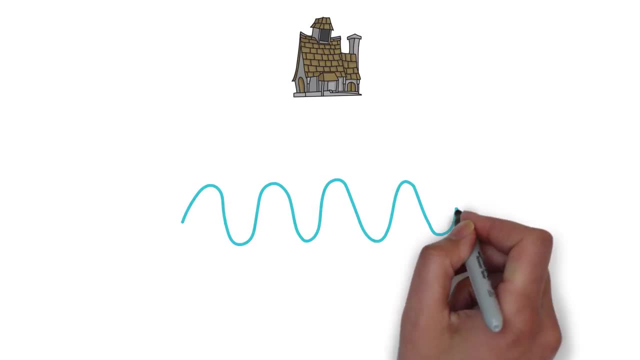 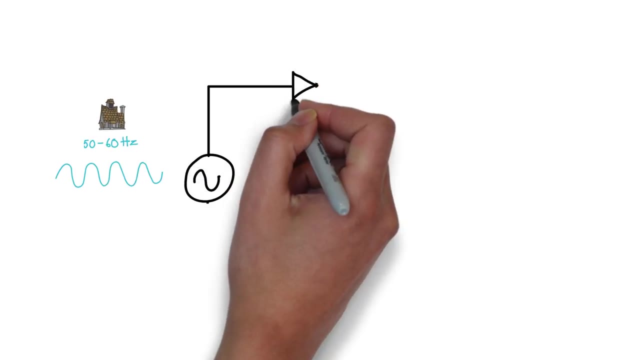 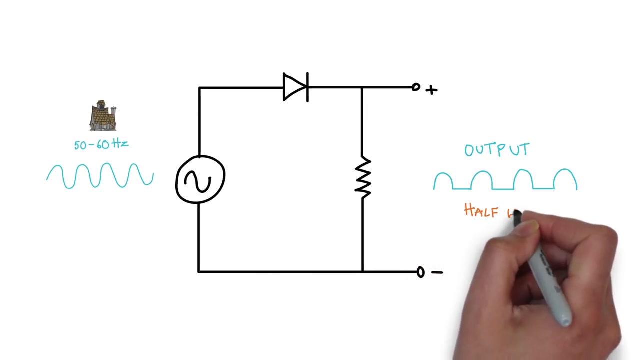 AC supply the voltage swings from positive to negative in cycle that repeat 50 to 60 times per second. Rectifier diode in series. with an AC voltage you eliminate the negative side of the voltage cycle and so end up with just positive voltage. This AC to DC conversion is called a half-wave. 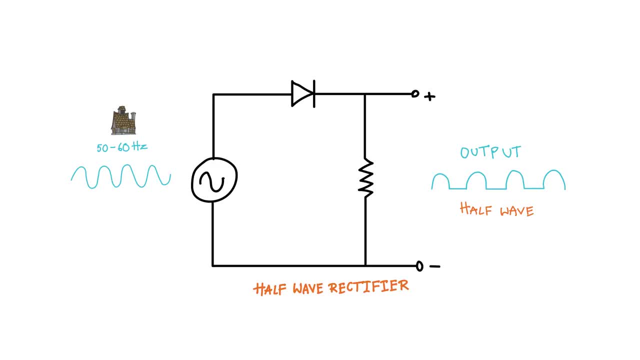 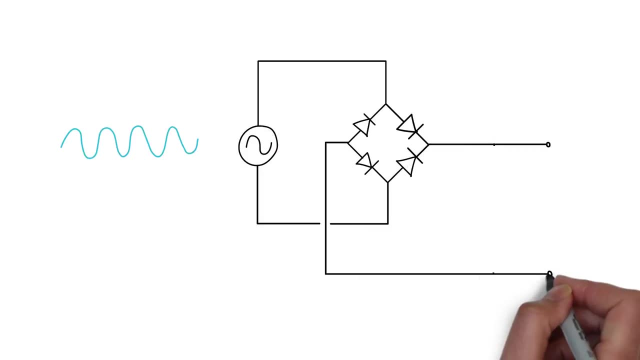 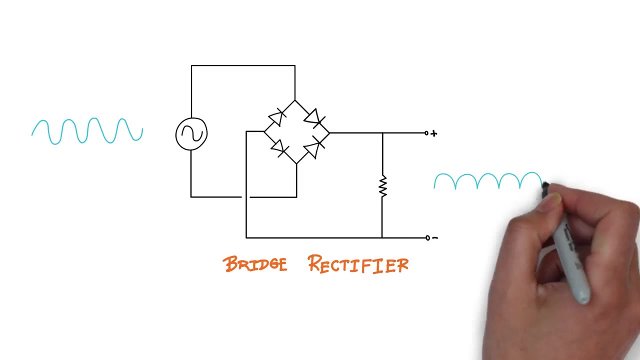 rectifier because it passes along only half of the incoming AC waveform. There's a better type of rectifier circuit that uses four rectifier diodes. This is called a bridge rectifier. A bridge rectifier is more efficient than a half-wave rectifier In the 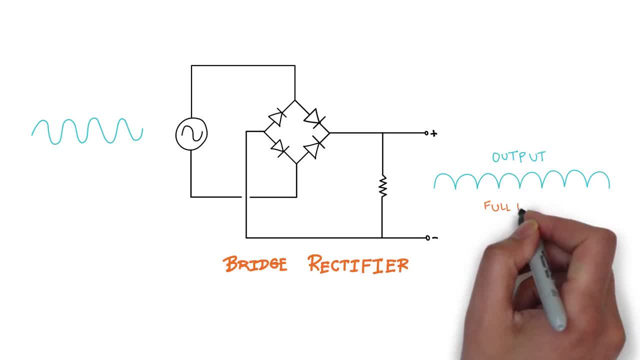 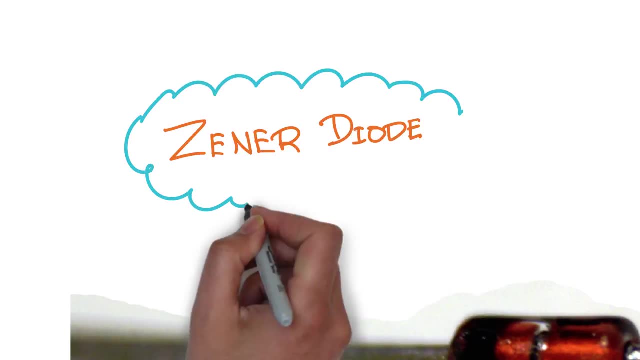 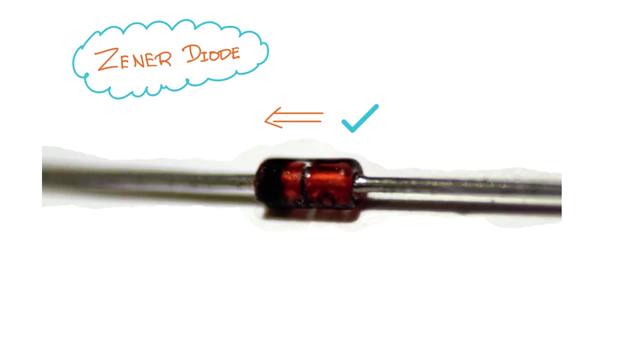 circuit. it allows both half of the AC wave to pass through. The negative half of the wave is inverted, so it becomes positive. A Zener diode generally behaves very similarly to a signal or a rectifier diode, except that its breakdown voltage is lower. A Zener diode is intended to allow current to flow when 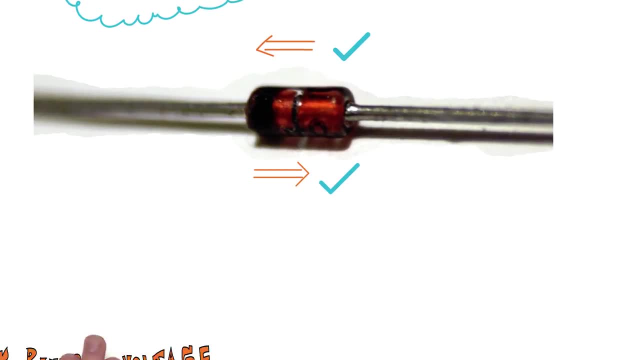 the peak reverse voltage is reached or exceeded. The peak reverse voltage of a Zener diode is called Zener voltage. As you can see, the schematic of a Zener diode is a bit different. It's a bit different from the schematic of. 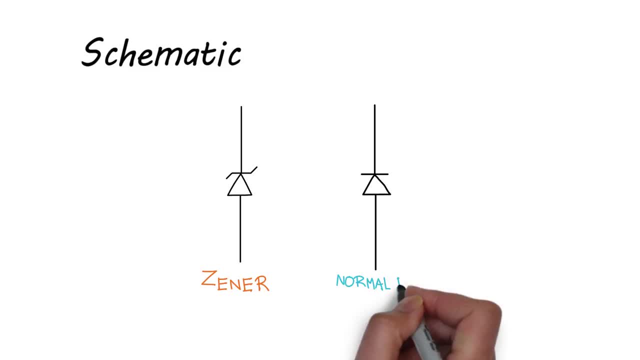 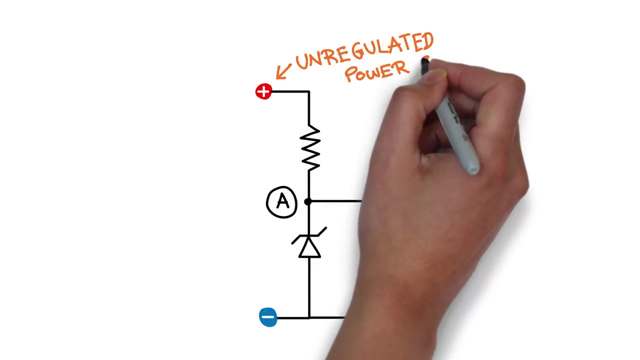 a Zener diode. The unique behavior of the Zener diode makes it usable as a very simple voltage controller when placed in series with a resistor. This is a simplified basic circuit illustrating the ability of a Zener diode to compensate for variation in the power supply or load. 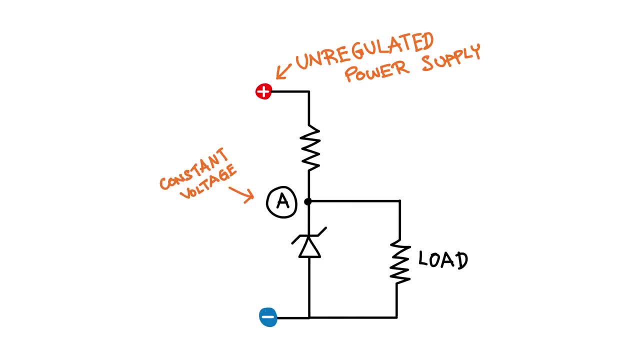 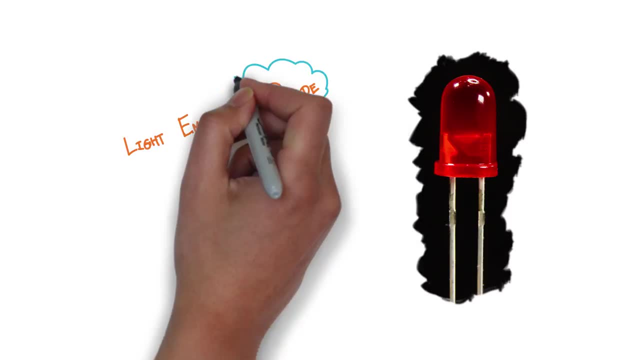 in a circuit creating an approximately constant voltage at point A. A light-emitting diode or LED is used to control the current of the Zener diode. A diode or LED is a special type of diode that emits visible light when current pass. 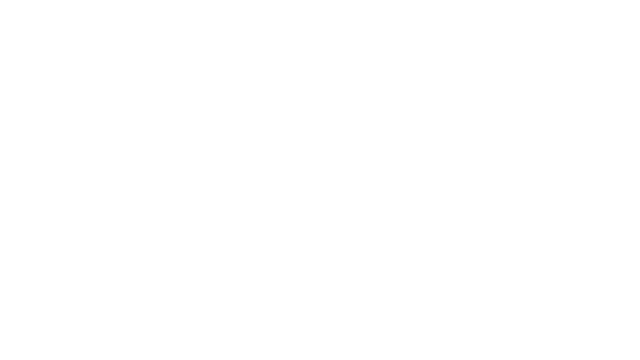 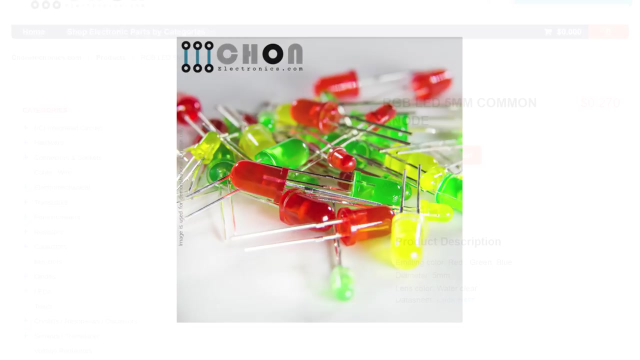 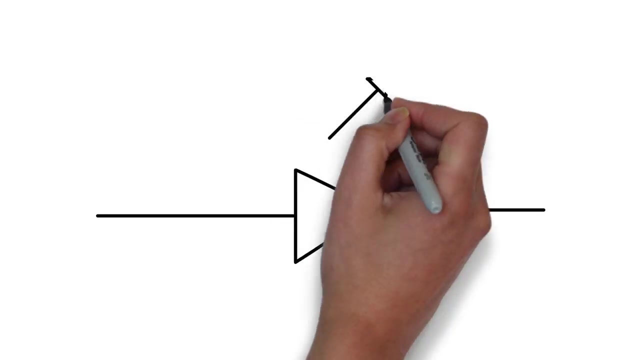 through it. LED come in variety of color, such as red, green, blue, yellow or white. There's also RGB LED that can bind red, green and blue into a single package. Here is the schematic of a LED. A LED is almost always connected in series with a resistor. 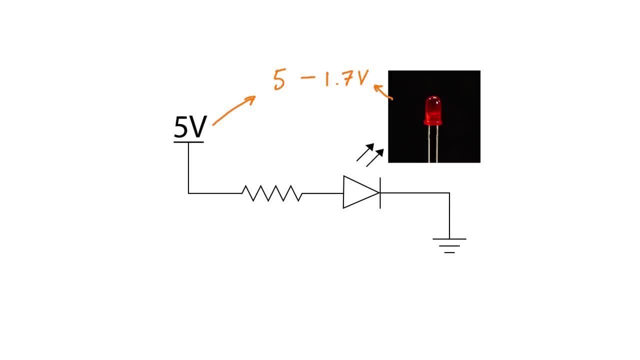 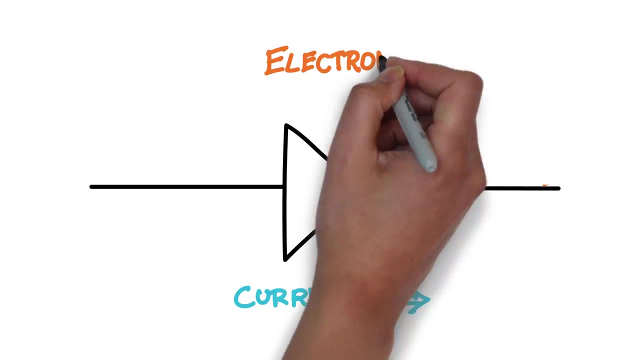 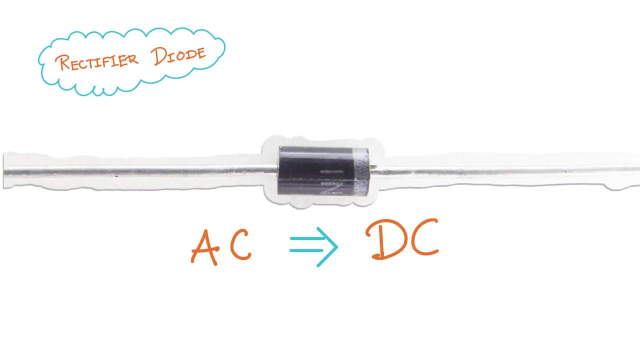 to protect the LED from damaging. Check out my resistor video on how to calculate the resistor value to be used with a LED. That's all for today. If you want to see more videos on the subject of electronics, please subscribe or leave a comment. See you next time.